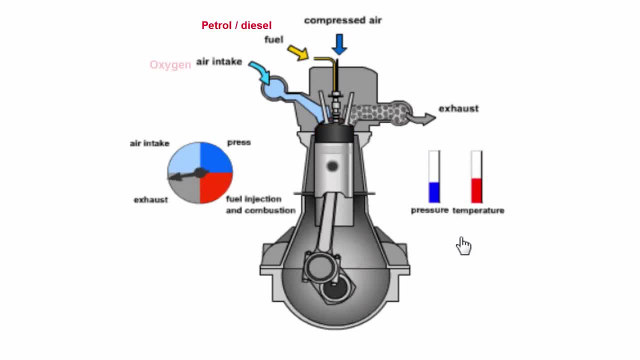 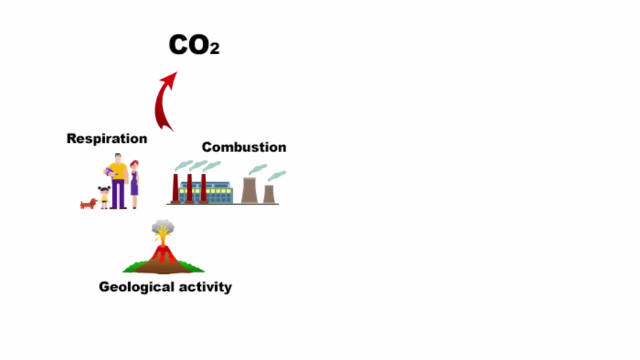 process in which substances like petrol, diesel reacts with oxygen to produce heat. Again, even here, carbon dioxide, and carbon monoxide is a byproduct. So anyway, whether it is respiration or combustion, carbon dioxide is released into the atmosphere. Once the carbon dioxide is out, 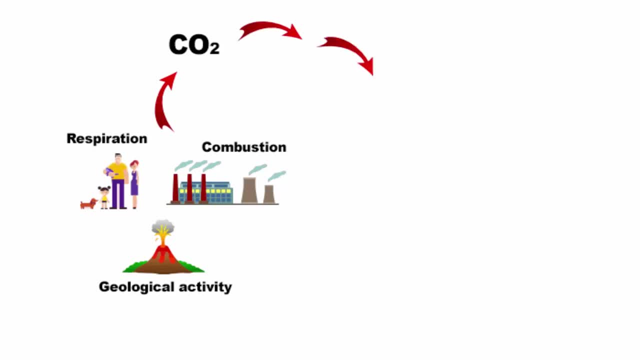 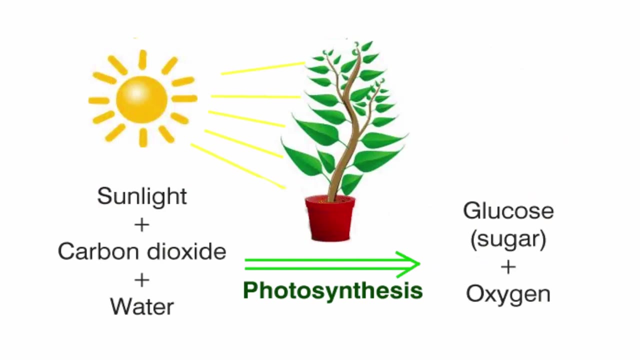 there in the atmosphere. the next step is the entry of the carbon dioxide in the photosynthetic process. When we say the word photosynthetic, immediately think of plants, trees and algae, Because trees and plants consume carbon dioxide and release oxygen. So basically the trees and 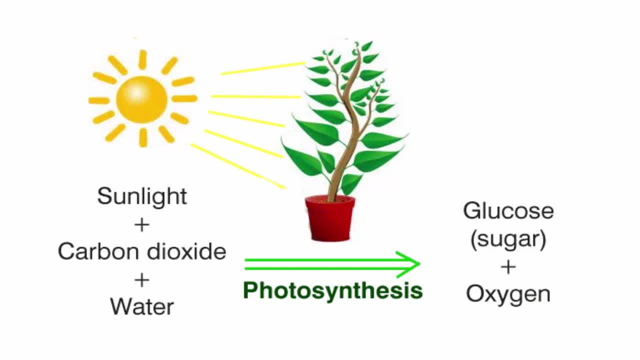 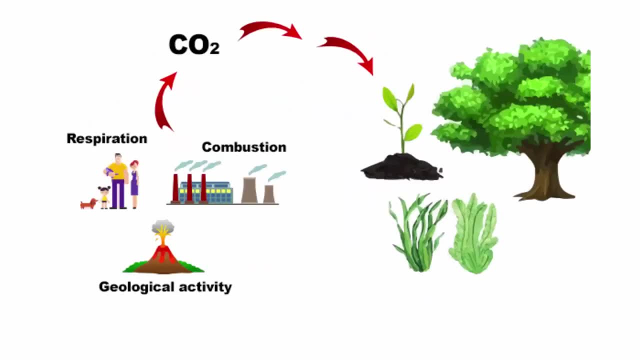 plants use energy to reproduce. It is done by taking in carbon dioxide and releasing oxygen. Look at this amazing part of nature. On one hand, the human being and mechanical devices have a certain way of functioning, And then, on the opposite side, there are trees, plants, algae. 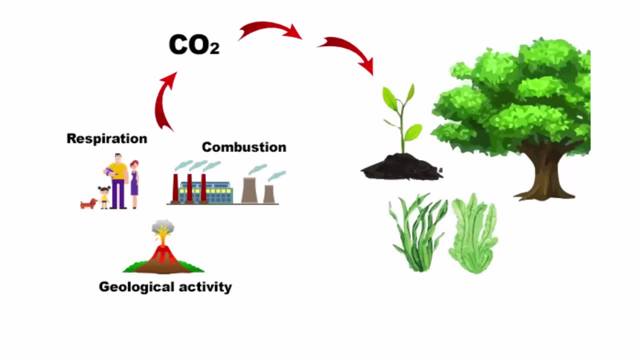 even they have their own way of doing things, which is completely opposite to us. You see, there is a fine balance between the two, And when we look at the picture, we see that the patient rocked into the fire. Of course there are trees, plants and algae, But 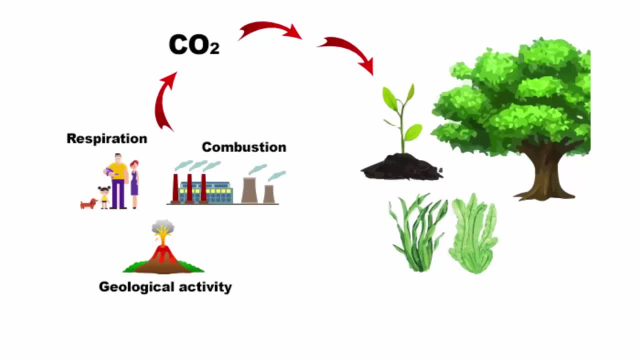 what does this mean? What is the question? So what is the problem here? Now? you got to utilise the image of a carbon dioxide to generate allowances in the��다 to destroy us. you get to see that carbon dioxide was already the most powerful and most pushy. 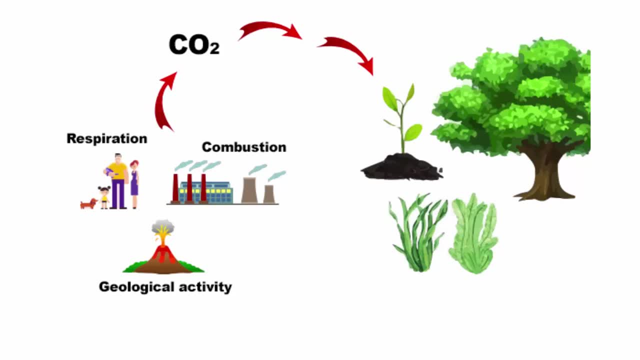 form of the self. With the help of the light cities, it is possible to cut its ends, and you upset all of our guards and guards who will keep on trying to find food or even the stench. Well, you see here. all of this is therefore complicated, As I checked out. 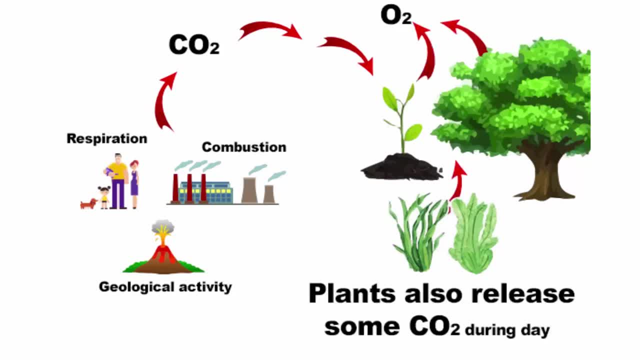 latest documents. I just got to this concept- more about the history right, where you can see the reason that even plants in the air cannot grow. Well, that means that plants- plants- can actually grow. So let us start with a term: ionising. 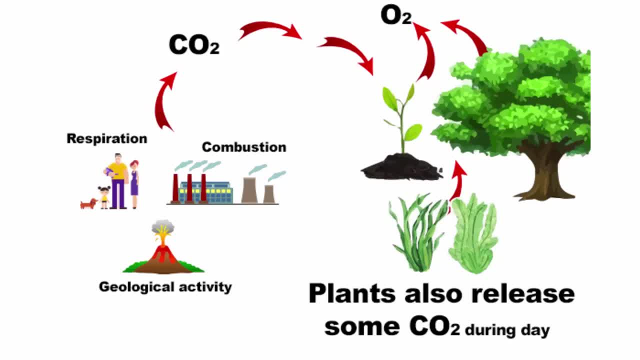 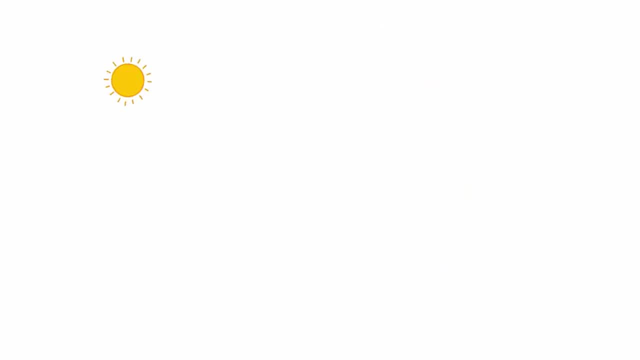 Now some of the carbon dioxide is released through its leaves and roots during the day. Then most of the carbon dioxide is contained within the plant tissue. Now, if you can recollect the ecological pyramid in that we have read that plants, trees and 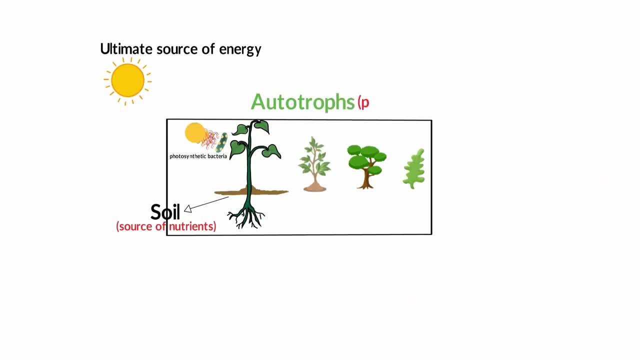 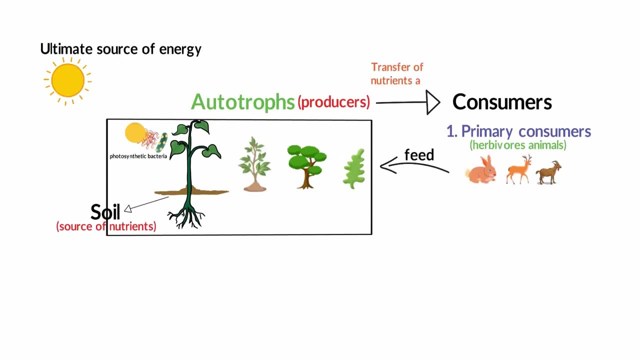 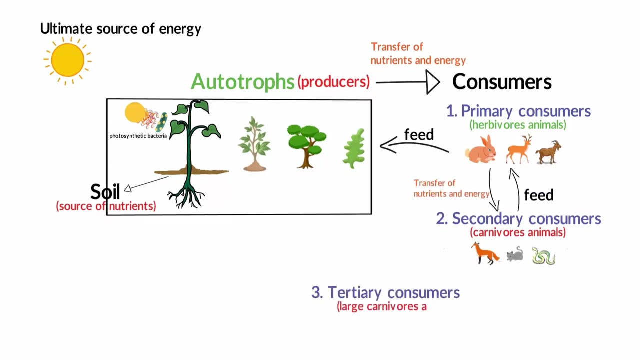 algae are called producers, And herbivorous animals feed on these producers for food and energy. When an animal consumes plants, the carbon compounds from the plant enters into the animal And then, in the final step, when plants and animals die, bacteria and fungi feed on the. 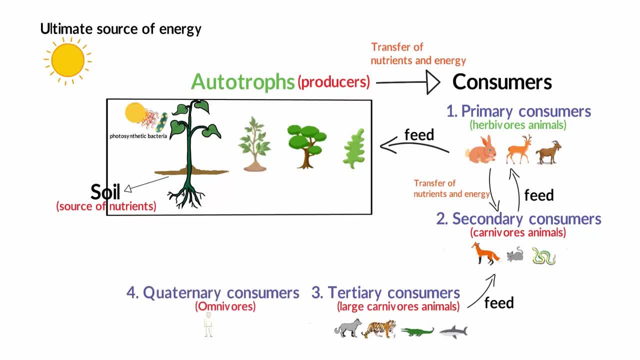 decays of dead plants and animals. This process is called decomposition, And again the by-product is carbon, which returns to the atmosphere. This entire cycle is called as carbon cycle.